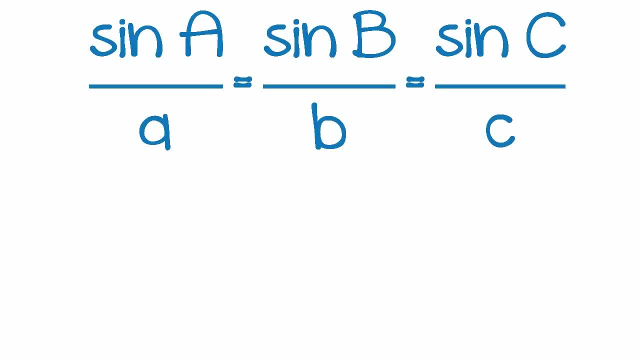 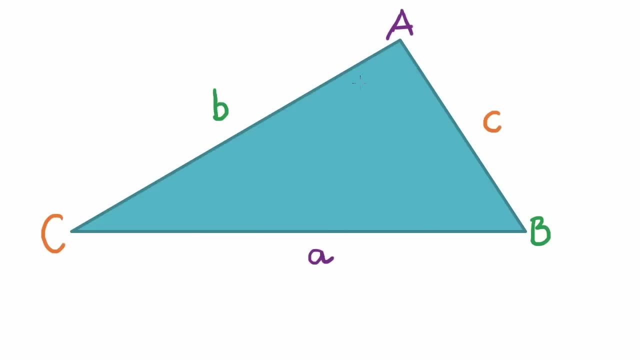 as sine a over a, equals sine b over b, equals sine c over c. Or you can flip those over if it suits you to do so, and you can write it as a over sine a equals b over sine b. So what's that telling us? Well, conventionally, when we label a triangle, if we call this angle up, 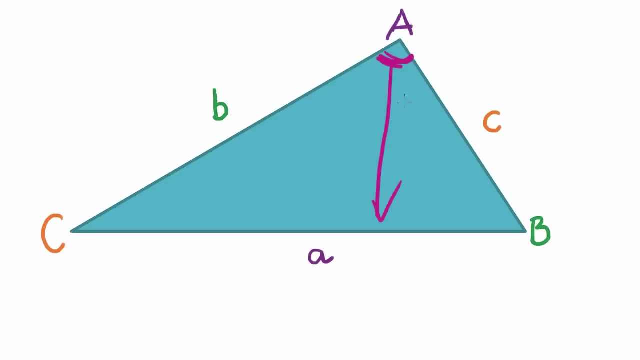 here a- this vertex a- then the side that it creates when that angle splays out and creates a line going along. here we call that little a. If we call this angle down here b- this vertex is b- then the line that it creates, splaying out to the other side all the way over here. 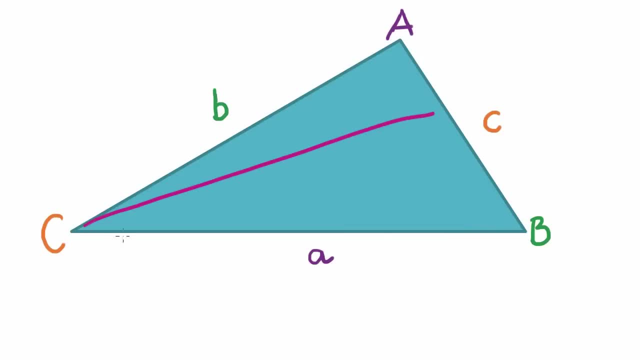 we call that little b And the same for c. This angle creates this line over here, so we call that capital C for the angle and little c for the line, and these you could think of as matching sets. so if we know that angle and down, 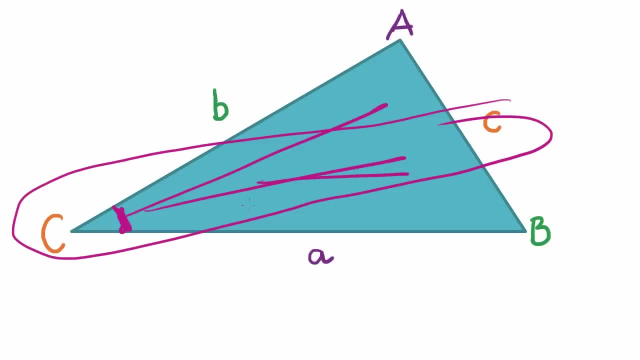 here. this angle C and the line that it creates those two pieces of information are correlated to one another. they kind of have something to do with each other, because how big or small the angle is like, if that was a much wider angle C- the line opposite- it would be much longer right, and if it was a skinny. 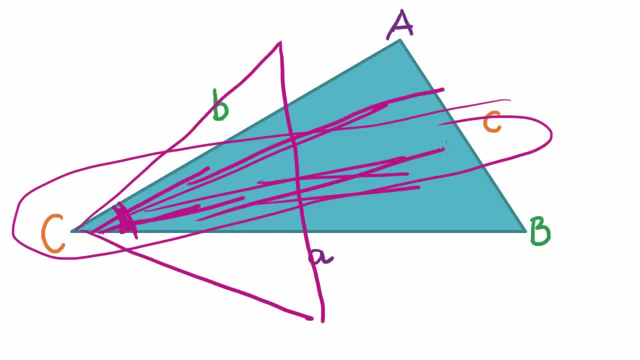 angle, then the line opposite. it would be really short coming out to here. so how fat or thin the angle is determines how long the line is. so they match. same with big A & little a. that's a matching set. and same with big B & little b. 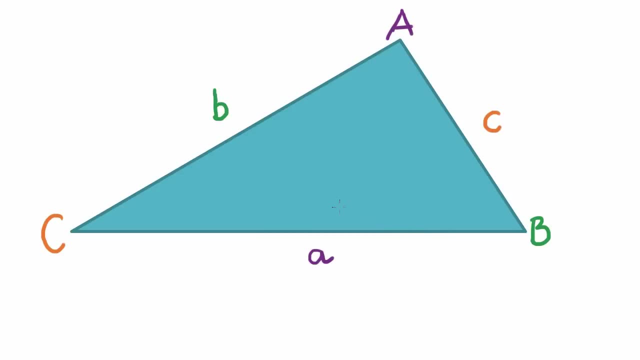 that's a matching set. now for the law of signs. to help us out, we need to know to matching sets because if we know B and little b and one of the two pieces of information that make up a and little a, so, for example, say, we know the angle. 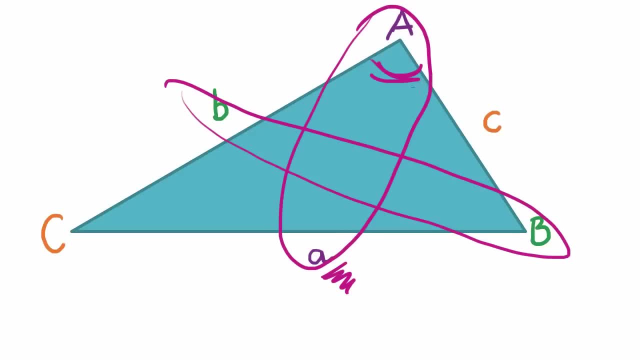 but we're trying to find the side, or we know the side and we're trying to find the angle. then, when we have two matching sets, there's four bits of info in that there's b over the sine of b and there's little a over the sine of a. now, if we have three of those pieces of information for 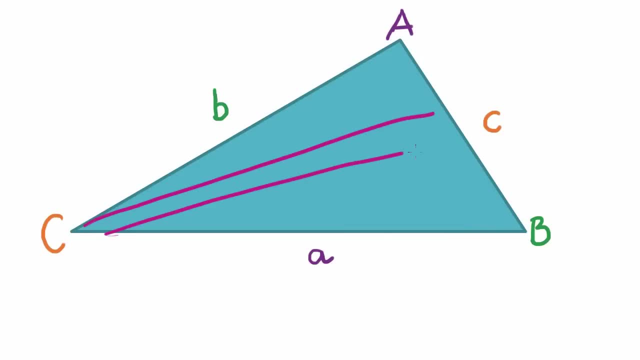 little b And the same for c. This angle creates this angle, this angle creates this angle, this line over here. so we call that capital C for the angle and little c for the line, And these you could think of as matching sets. So if we know that angle and down here this angle c and the 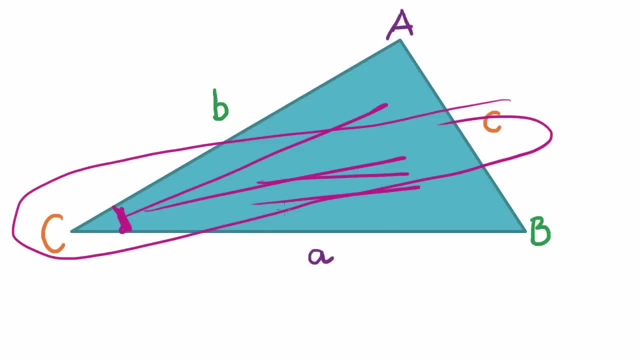 line that it creates. those two pieces of information are correlated to one another. They kind of have something to do with each other, Because how big or small the angle is like, if that was a much wider angle c the line opposite, it would be much longer right. 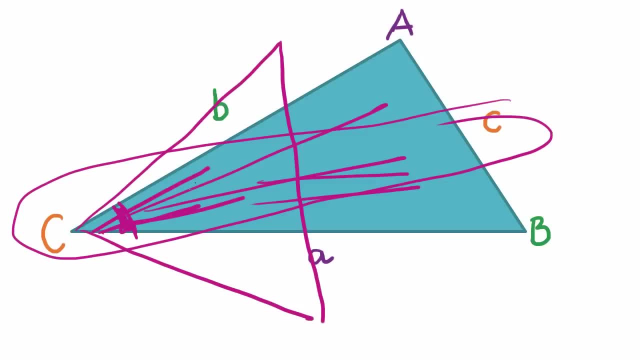 And if it was a skinny angle it would be much longer right, And if it was a skinny angle then the line opposite, it would be really short coming out to here. So how fat or thin the angle is determines how long the line is. So they match Same with big a and little a. That's a matching. 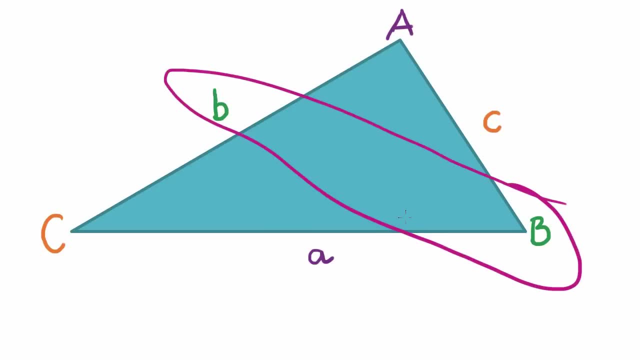 set And same with big b and little b. That's a matching set. Now for the law of science to help us out. we need to know two matching sets, Because if we know b and little b and one of the two pieces of information that make up a and little a. so, for example, 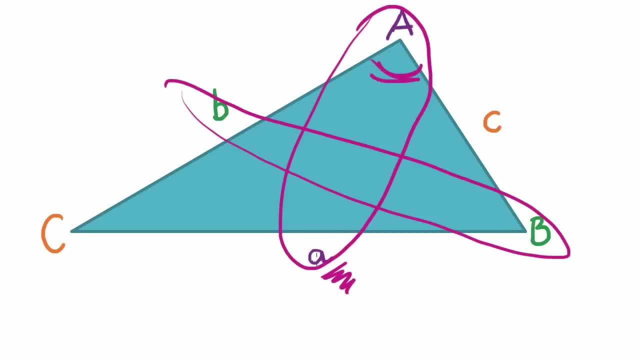 say: we know the angle but we're trying to find the side, or we know the side and we're trying to find the angle. then, when we have two matching sets, there's four bits of info in that There's b over the sine of b and there's little a over the sine of a. Now, if we have three of those, 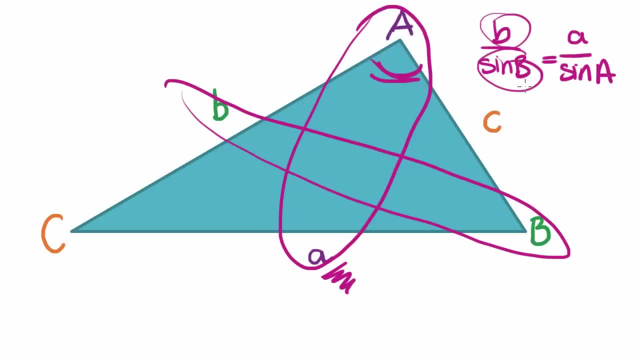 pieces of information, for example little b, sine of b, and we don't know little a. that's an unknown, but we know sine of a, for example. then we can work out the rest. So essentially, what you need to make the sine rule work for you is to know one complete matching set, That is 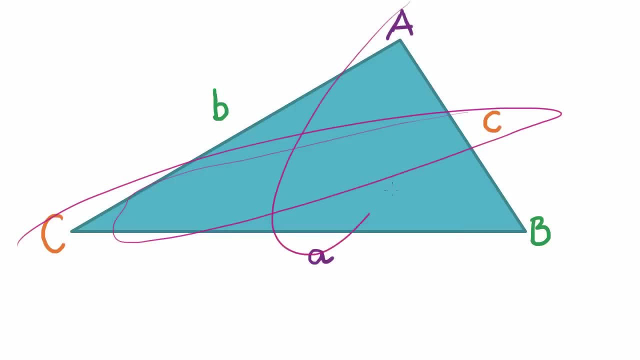 either c and little c or a and little a or b and little b. You need one complete matching set and then one half-filled out matching set. So one piece of information about somewhere else, and we'll use its corresponding matching set side to figure out the rest. Let me show you. 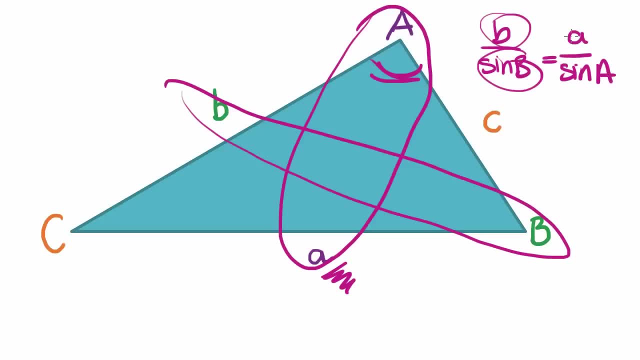 example, little b, sine of b, and we don't know little a. that's an unknown, but we know sine of a, for example. then we can work out the rest. so essentially, what you need to make the sine rule work for you is to know one complete matching set, that is, either you know c and little c, or a and 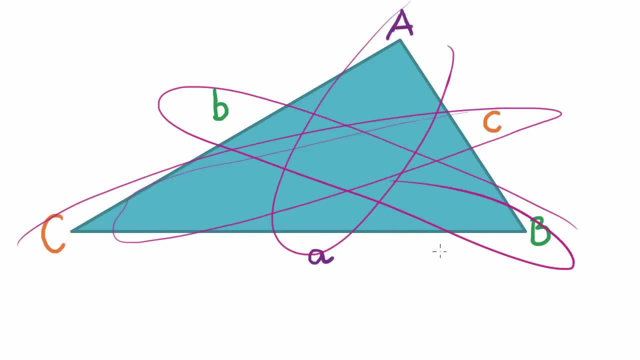 little a or b and little b. you need one complete matching set and then one like half filled out matching set. so one piece of information about somewhere else and we'll use its you corresponding matching set side to figure out the rest. Let me show you what I mean. So here's an example In this. 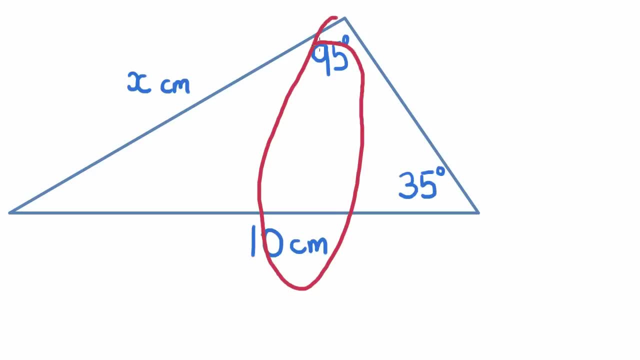 non-right angle triangle. we have a matching set here of 95 degrees and 10 centimeters, and we have a matching set here with 35 degrees and our unknown, which is this side along here. Now I could choose to write sine A over A equals sine B. 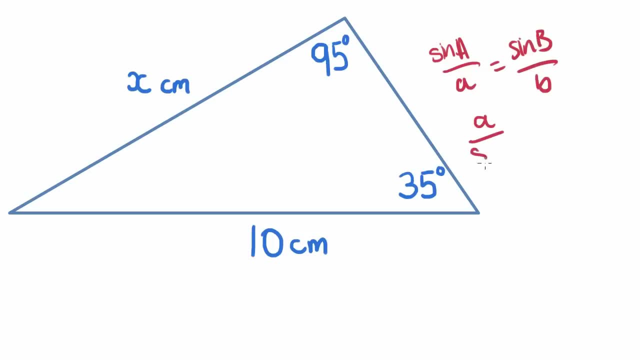 over B, or I could choose to write A over sine. A equals B over sine B. The way I'm going to choose which way to write it is I'm going to put my unknown on the top of the equation and put it on the numerator, because it just means you have less algebra. 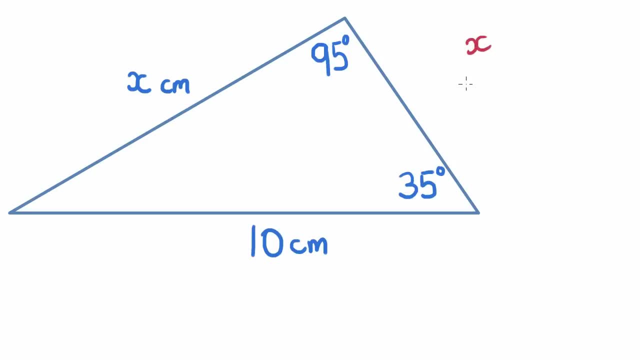 to do later on. So my unknown is X and that's a side. I'm going to put that here, and it's going to be over the sine of its matching partner. Now its matching partner is 35 degrees, so it's over sine of 35.. Now the corresponding piece of information that I'm going to use. 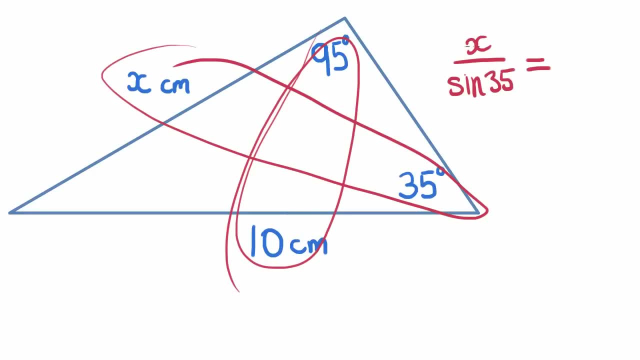 is this other matching set that I have. I just need to put them in the same order. so I have sides over angles. So I'm going to put the side 10, over sine of the angle, which is 95. And now to get the X by itself, I'm going to times the sine 35 over to the other. 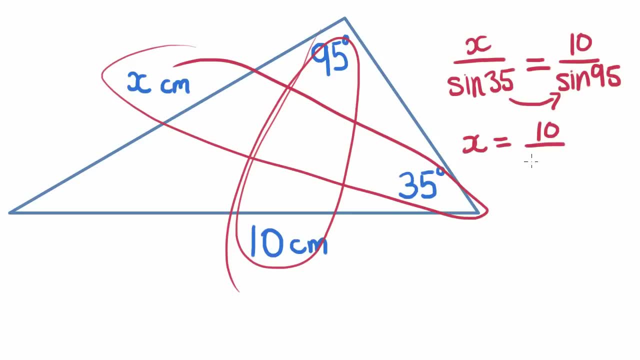 side of the equals. I have X equals 10 divided by sine of 95 times sine of 35.. Enter that into your calculator and you get X equals 35.. that into your calculator and you get x equals 5.76 centimetres. Now what would happen if they? 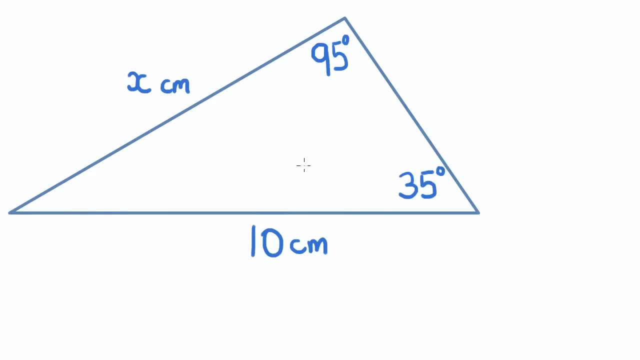 what I mean. So here's an example: In this non-right angle triangle we have a matching set of ninety-five degrees and ten centimeters, and we have a matching set here with thirty-five degrees and our unknown, which is this side along here. Now I could choose to write sine. 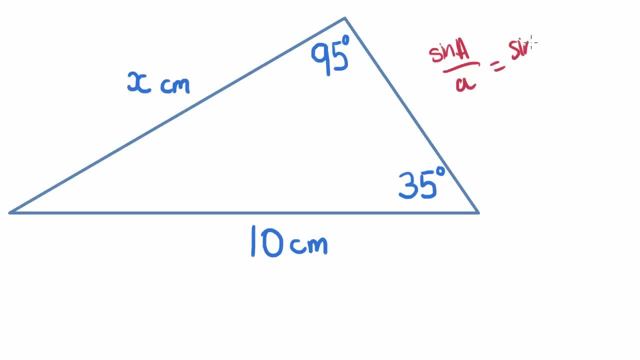 a over a equals sine b over b. or I could choose to write a over sine a equals b over sine b. The way I'm going to choose which way to write it is: I'm going to put my unknown on the top of the equation. I'm going to put it on the numerator. 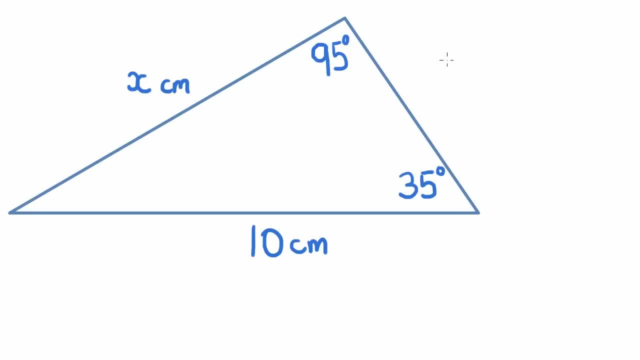 Because it just means you have less algebra to do later on. So my unknown is x and that's a side. I'm going to put that here, and it's going to be over the sine of its matching partner. Now its matching partner is thirty-five degrees, so it's over sine of thirty-five. 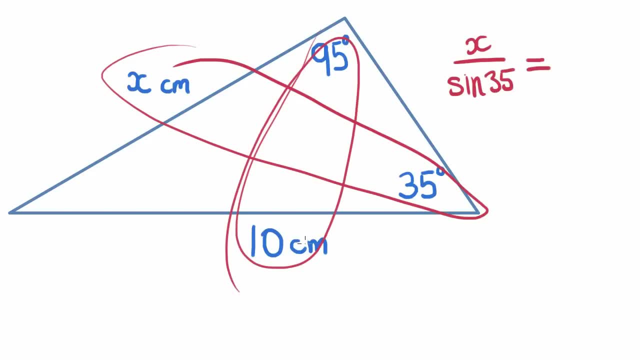 Now the corresponding piece of information that I'm going to use, this other matching set that I have. I just need to put them in the same order. So I have sides over angles, So I'm going to put the side ten over sine of the angle, which is ninety-five. So that's. 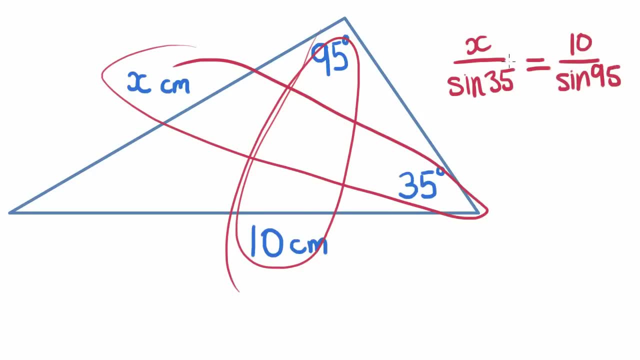 thirty-five. And now to get the x by itself, I'm going to times the sine thirty-five over to the other side of the equals. I have x equals ten divided by sine of ninety-five, times sine of thirty-five. Enter that into your calculator and you get x equals five. 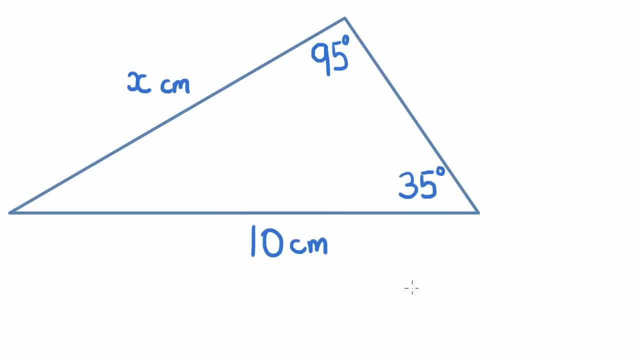 point seven, six centimetres. Now, what would happen if they hadn't given us this piece of information down here, this thirty-five, Let's say that we were given this one instead, which is fifty degrees. Now can we use the sine rule? We still have our matching set here, which is going to help us out, but now, 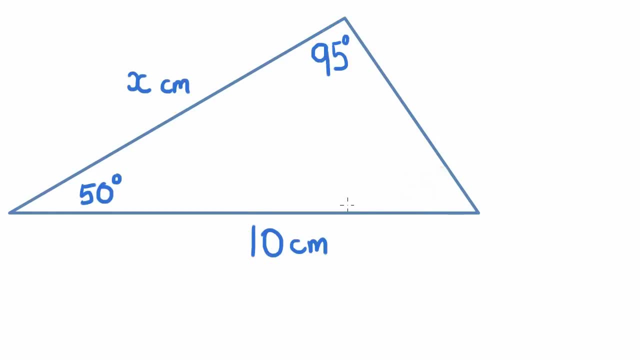 we don't know what's opposite, the x, so that's a bit of a problem, But remember how all the angles in a triangle add up to a hundred and eighty degrees. There isn't much maths that we have to do before we can figure out what this angle is. All we need to do is a hundred. 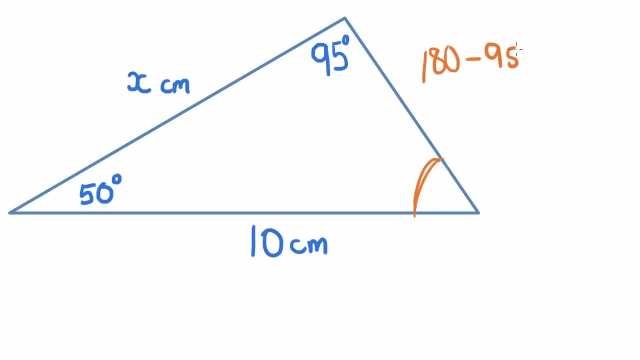 and eighty minus ninety-five minus fifty, and we get an answer of thirty, Thirty-five degrees, And then we can use this matching pair to do the sine rule. So if you don't see a matching pair straight off the bat, just have another quick look. 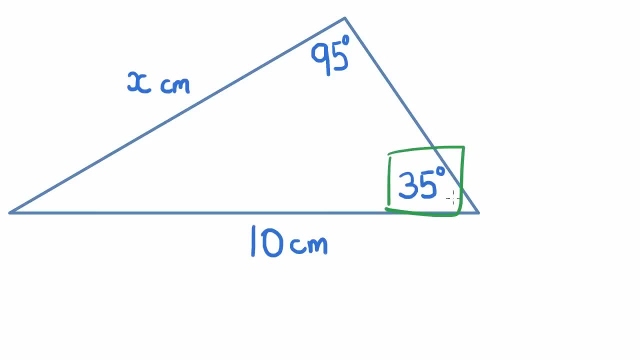 hadn't given us this piece of information down here, this 35?? Let's say that we were given this one instead, which is 50 degrees. Now can we use the sign rule? We still have our matching set here, which is going to help us out, but now we don't know what's opposite the x, so that's a bit of a. 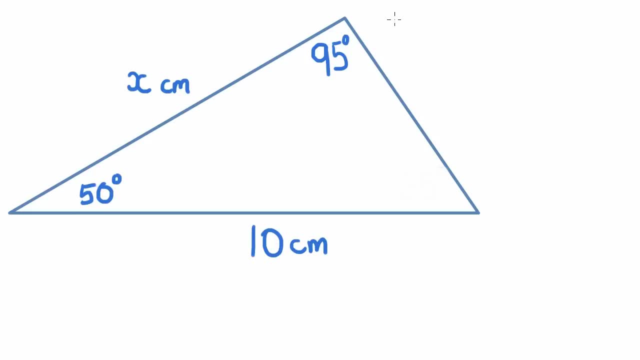 problem, But remember how all the angles in a triangle add up to 180 degrees. There isn't much maths that we have to do before we can figure out what this angle is. All we need to do is 180 minus 95 minus 50, and we get an answer of 35 degrees, and then we can use this matching pair. 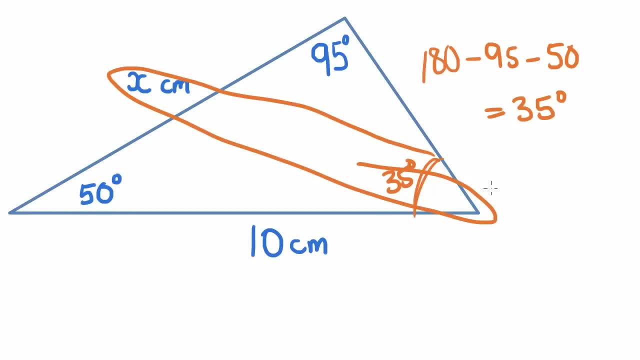 to do the sign rule. So if you don't see a matching pair straight off the bat, just have another quick look and see if you can work it out easily. What if, for this question, they had told us that this was 5.76 centimetres, but they had asked us to? 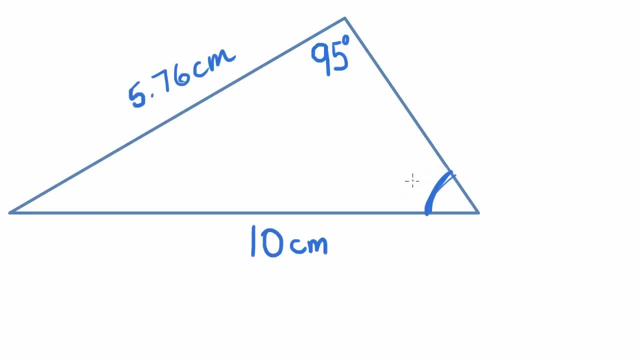 find what this angle was down here. This was an unknown angle, theta. We'd go about this in much the same way. it's just we'd be flipping our sign rule the way we write it out, So we're going to use this matching piece of information here. This matching set will help us out, and this is our. 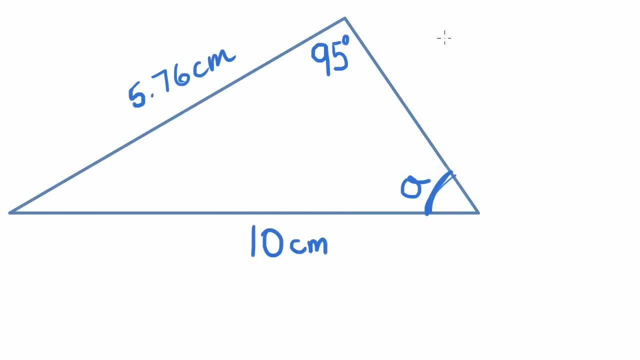 matching set that includes an unknown. Now I'm going to write the unknown on the top. so I'm going to have theta and theta. So I'm going to have theta and theta. So I'm going to have theta, that unknown, divided by its side, which is 5.76, and that's going to be equal to the other matching. 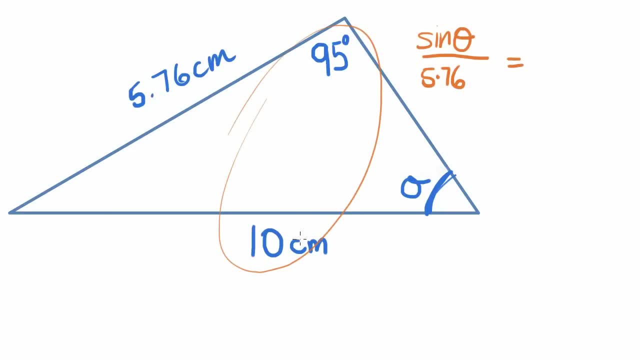 set. Now. this time I have angles on the top and sides on the bottom, So I'm going to have sine of 95, because we want the sine angle both on the top or both on the bottom. That's divided by 10.. Now 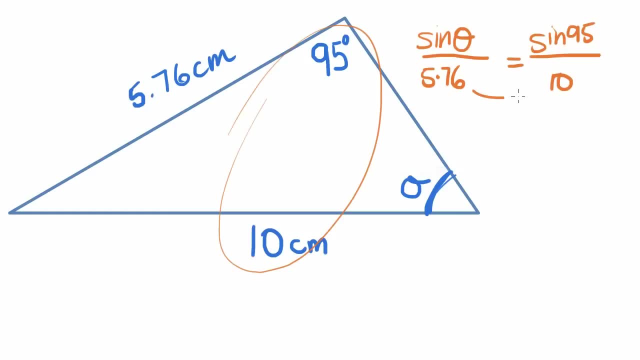 to get this 5.76 over to the other side, I'm going to multiply it over there. So I end up with sine theta equals sine of 95 divided by 10 times 5.76.. Now to undo the sine business over here. 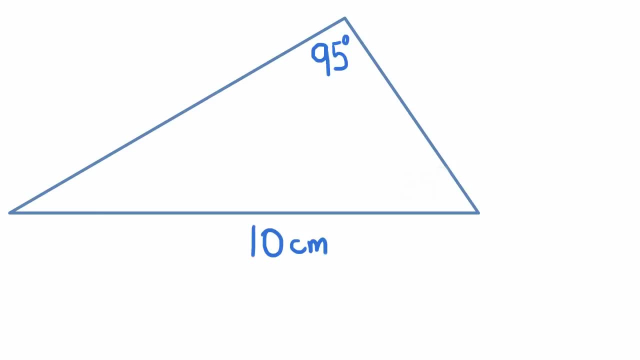 and see if you can work it out easily. What if, for this question, they had told us that this was five point seven, six centimetres, but they had asked us to find what this angle was down here? This was an unknown angle, theta. We'd go about this in much the same. 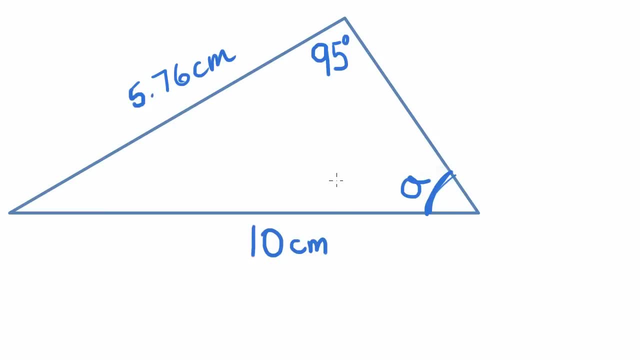 way It's just we'd be flipping our sine rule the way we write it out. So we're going to use this matching piece of information here. This matching set will help us out, and this is our matching set that includes an unknown. Now I'm going to write the unknown on the top, So I'm going to have 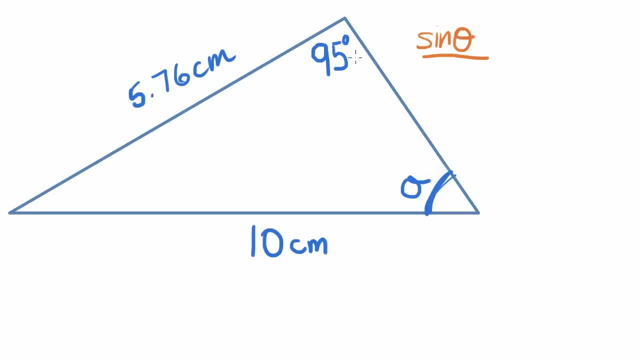 sine of theta, that unknown, divided by its side, which is five point seven, six, and that's going to be equal to the other matching set. Now, this time I have angles on the top and sides on the bottom, So I'm going to have sine of ninety-five, because that's going. 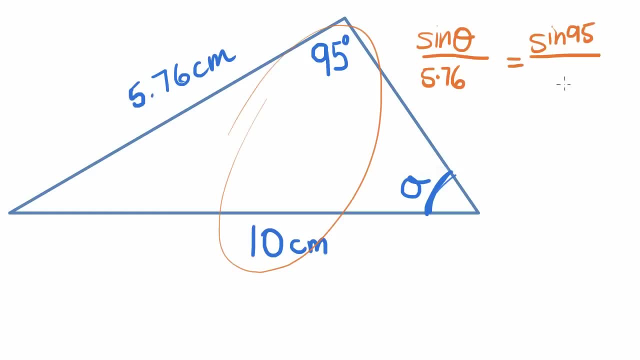 to be five point seven six, because we want the sine angle both on the top or both on the bottom. That's divided by ten. Now to get this five point seven six over to the other side, I'm going to multiply it over there, So I end up with sine theta equals. 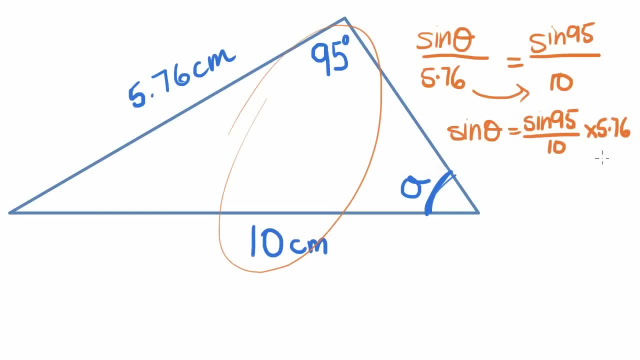 sine of ninety-five divided by ten times five point seven, six. Now to undo the sine business over here. basically, what I'm going to do, the inverse of that operation, is to take the inverse sine. So theta equals the inverse sine over here and that's going to be the. 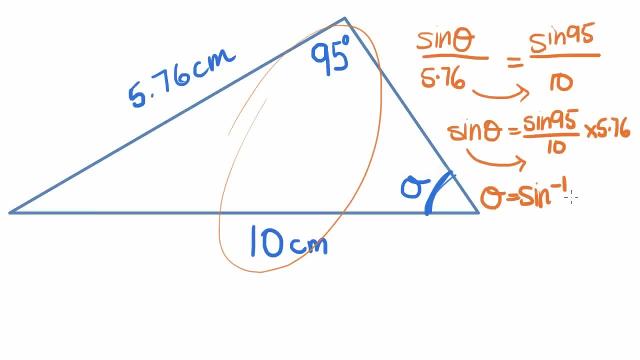 sine, which on your calculator looks like sine to the negative, one of all of this information. So when I work this out on the calculator, that gives me point five, seven, three, And now what I'm going to do is take the inverse sine. I'm going to hit sine to the negative. 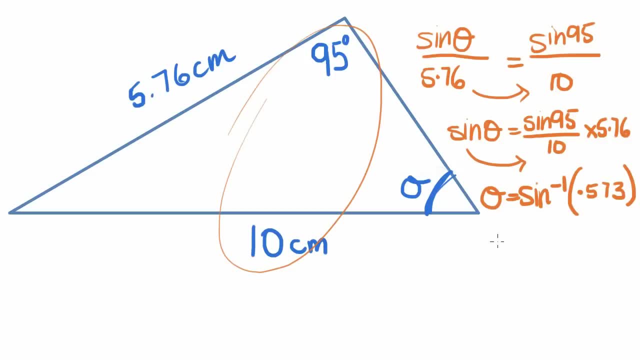 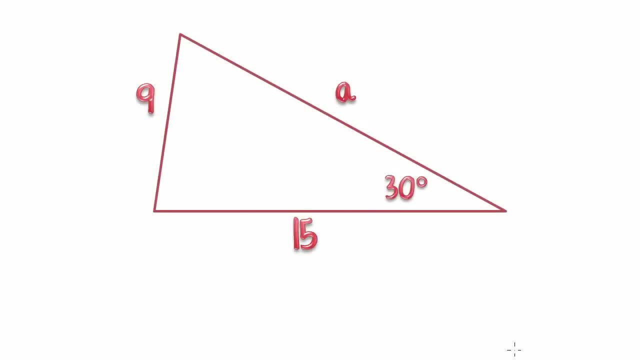 one of that point. five, seven, three And what do you know I end up with. theta equals thirty-five degrees. So in this example here I have a couple of matching sets, but they're not that obvious. First of all I have nine and thirty degrees. They match, But then the a over here is going. 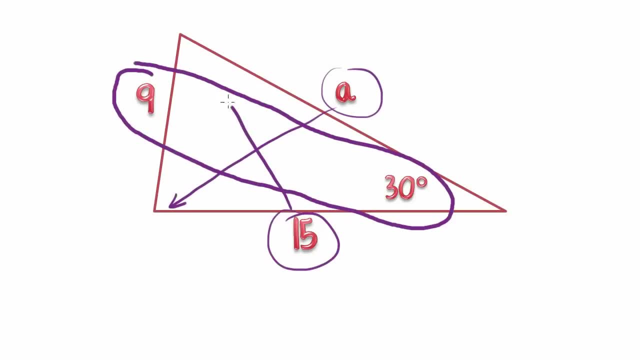 to correspond to that angle and the fifteen over here is going to correspond to that angle. So as yet I only have one matching set. So I can't work out a yet because I don't know what the angle that matches it is. But what I can work out is this angle up here because 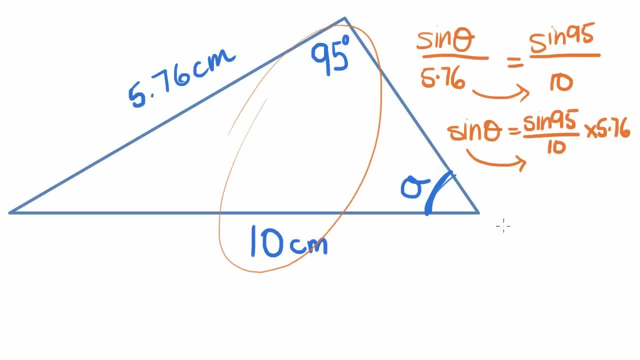 basically what I'm going to do. the inverse of that operation is to take the inverse sine. So theta equals the inverse sine, which on your calculator looks like sine, to the negative one of all of this information. So when I work this out on the calculator, that gives me 0.573. and now what I'm? 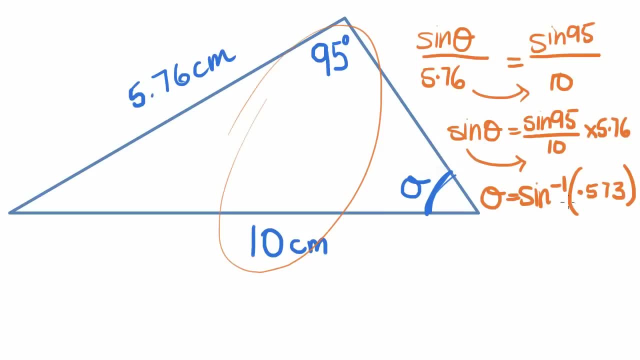 going to do is take the inverse sine and I'm going to take the inverse sine, and I'm going to take the inverse sine, I'm going to hit sine to the negative one of that 0.573, and what do you know? I end up. 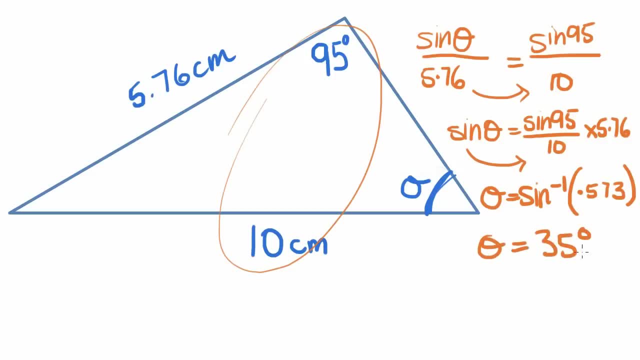 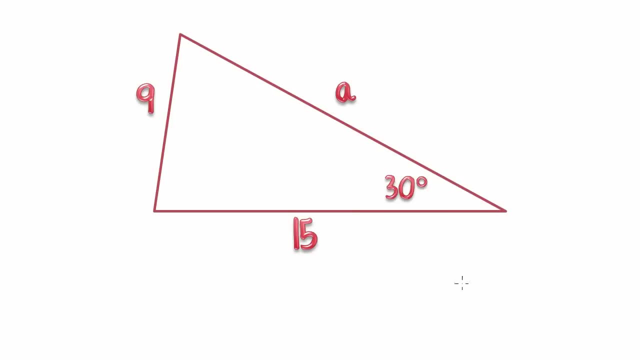 with theta equals 35 degrees. So in this example here I have a couple of matching sets, but they're not that obvious. First of all I have 9 and 30 degrees. They match, But then the a over here is going to correspond to that angle and the 15 over here is going to correspond to that angle. So as 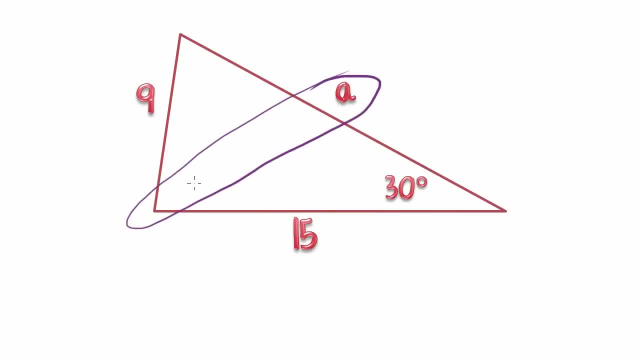 I said, I have this set of matching sets So I can't work out a yet because I don't know what the angle that matches it is. But what I can work out is this angle up here because I have 15 corresponding with it. So let's use sine of 30 over 9 and that is going to be equivalent to this. 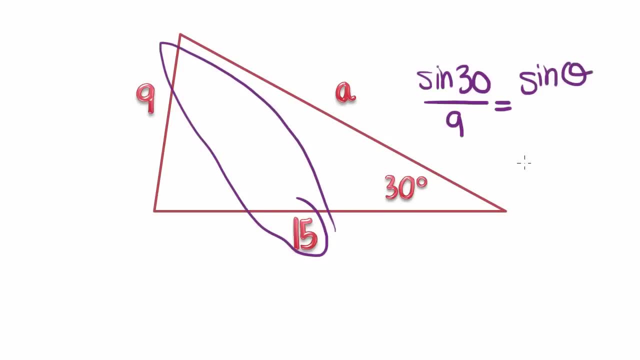 other matching set which is sine of- goodness knows, we don't know yet. let's call it theta over 15.. So how do we work this out? We times the 15 over to that side to get rid of it. We have sine of 30 over 9 and that is going to be equivalent to this other matching set which is: 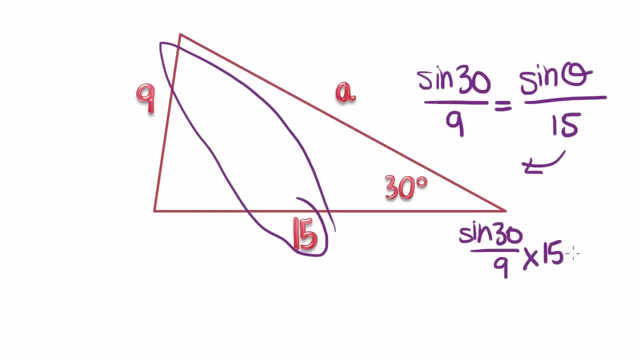 sine of 30 over 9 times 15 equals sine. of theta is 0.8333.. Now to get rid of the sine on that operation, to kind of put the do the inverse operation and get sine over to the other side, we take the inverse sine. So on your calculator that looks like sine to the negative 1 of 0.8333. 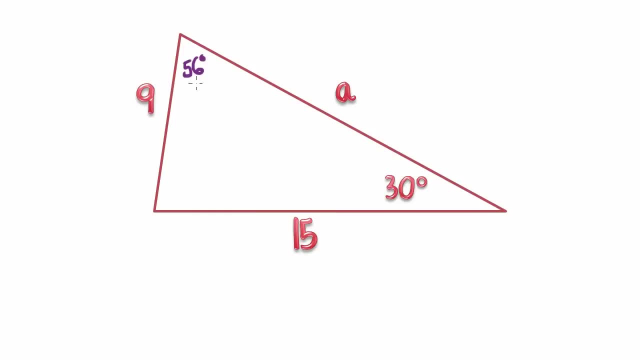 which is 56 degrees. Now that I know that, I can work out what this last remaining angle down here must be, because all of the angles in a triangle add up to 180.. So if I have 180 minus 30 minus 56, I have whatever is left over as this angle, So that's 94.. Now I have a